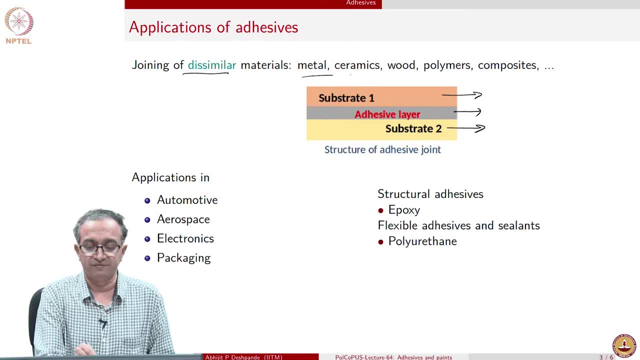 different types of joints are possible, So all different types of materials can be bonded together using adhesives. And why is this required? Because, rather than fabricating and using mechanical fastening or processes, which can be very expensive, what we could do is we do not have to worry about what material are we making things out of Once those components. 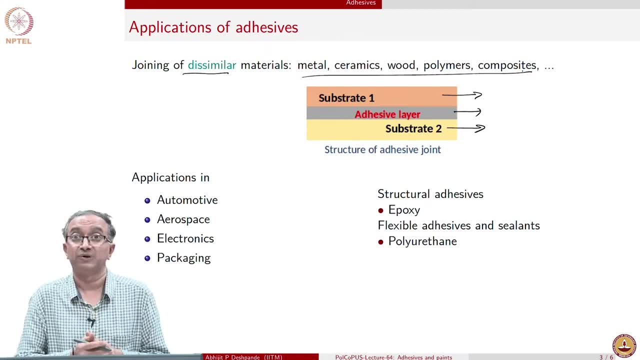 are made. you can use a third substance in which, in this case, is macromolecular adhesive. you can then bond any of those substances. So therefore, applications are everywhere in transport and total transport, Notice, by using an adhesive. these substances are not. 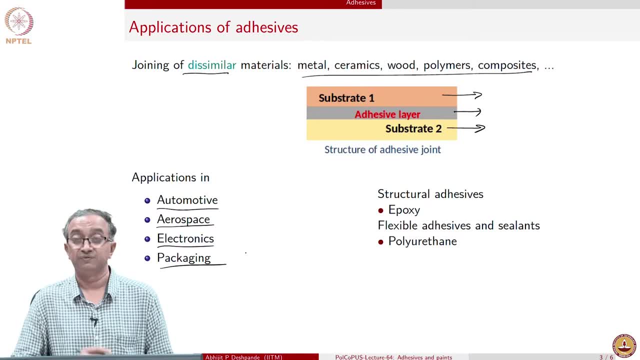 in electronics, in packaging- So various places we can use the idea of adhesive bonding And generally, if you look at structural adhesives, they are playing a structural role and therefore they are load bearing and the strength of the adhesive joint based on these. 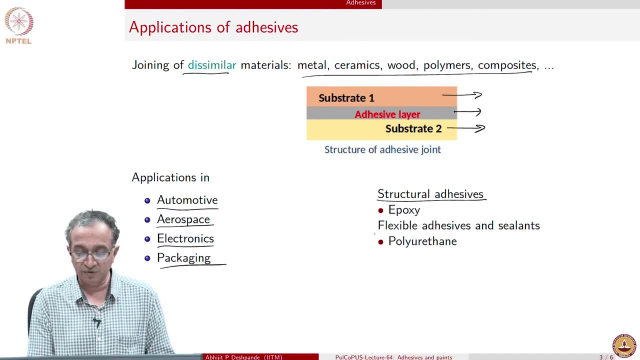 structural adhesives is extremely good, And we can also have flexible adhesives and sealants which play role of not only holding materials together, but they are not structural materials, but they do play a role of sealing where leakage cannot happen from one side to the other side. 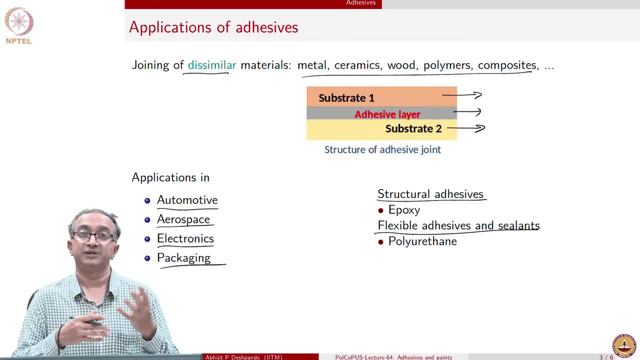 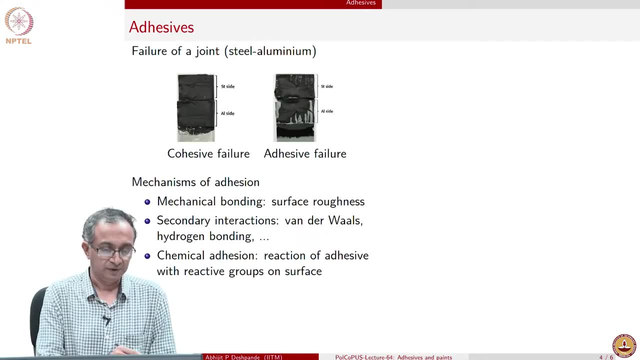 So therefore, these flexible adhesives play a role of vibration isolation, sealant, as well as holding the overall components together. So the key thing related to these adhesives is the fact that when we are bonding two surfaces with an adhesion- here, for example, there is a steel and aluminum- 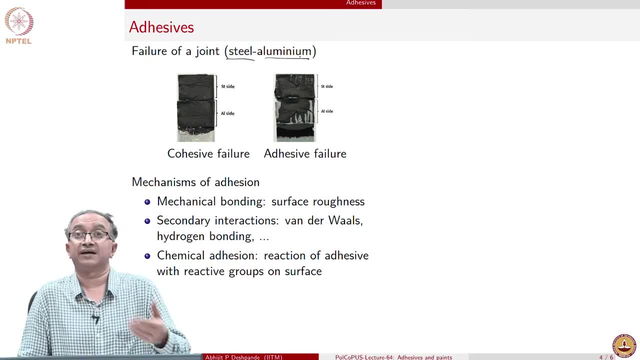 joint which is bonded using this black looking polyurethane adhesive, and then you can see the steel side and the aluminum side. So what has been done in this case is you take, let us say, steel and you take aluminum, and then in between you put the adhesive and you make a bond like 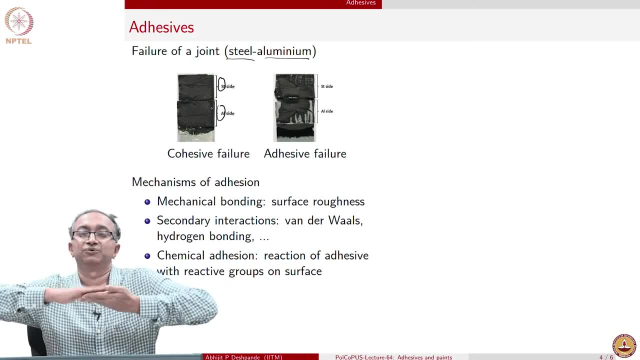 that, and then what you do is you pull it apart to see you know what happens. how does it fail? And if you then look at these two surfaces, if let us say there is a lot of adhesive here and lot of adhesive here, then what you have is a cohesive failure. So it is, adhesion was good. 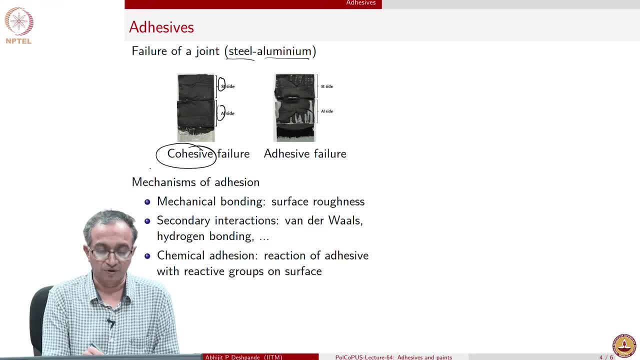 and because the adhesive failed. the joint failed, But you could also have the adhesive failure, in which case the adhesive did not really bond with the surface. So in this case you can see that the bonding with aluminum was not very good, because you can see exposed aluminum, You can 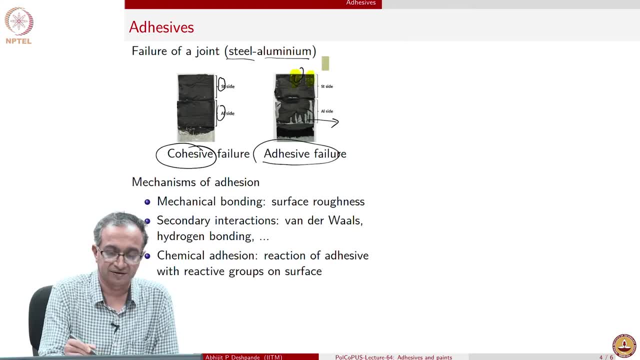 also see several places where the adhesive did not bond with the surface. So in this case you can see several places where there is exposed steel. So even bonding with steel was not good. So ideally, what you want is a process where the full strength of the adhesion is encountered by 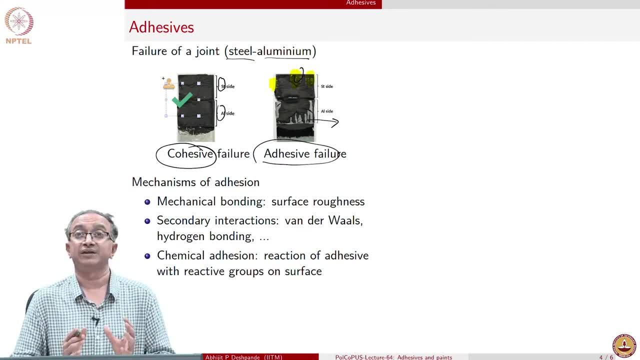 adhesive failure itself. So generally, how this can be ensured is when the adhesion with the surfaces has to be very good. So there has to be several mechanisms of adhesion which have to come together for us to give very good adhesive strength of the overall joint. So you can have 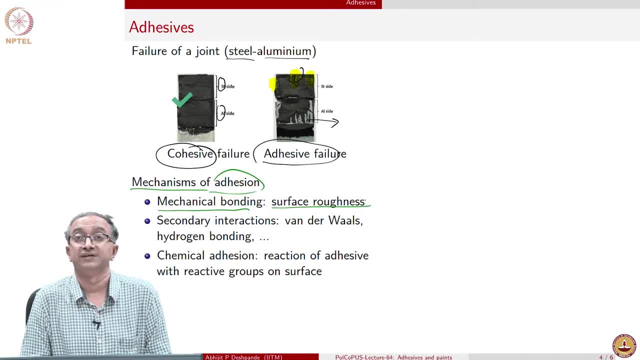 let us say mechanical bonding, which is induced because of surface roughness, Because the aluminum surface, let us say, is very rough and whatever is the macromolecular adhesives, it can go and basically interact with the metal surface in all of these rough. 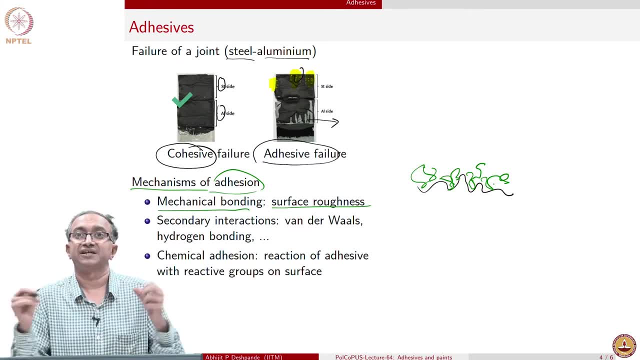 protrusions and valleys which are there on a metal surface. On the other hand, if we have a metallic surface, we can have a metal surface which is very rough. So we can have a metal surface which is very rough, So we can have a metal surface which is very smooth. Then the macromolecule will have less area to 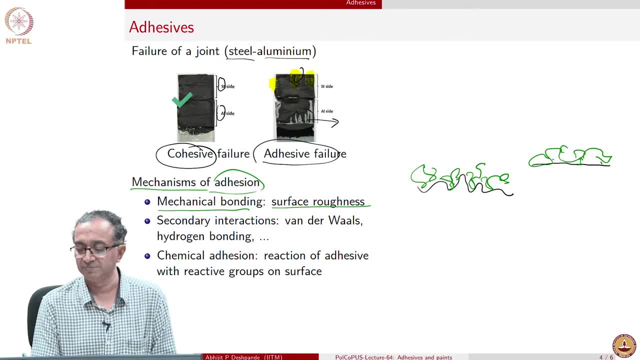 interact, and the number of points where the physical bonding may be there is much less. So this is something like mechanical interlocking between two materials, And of course the interactions between the metal atoms and the macromolecule has to be very good in. 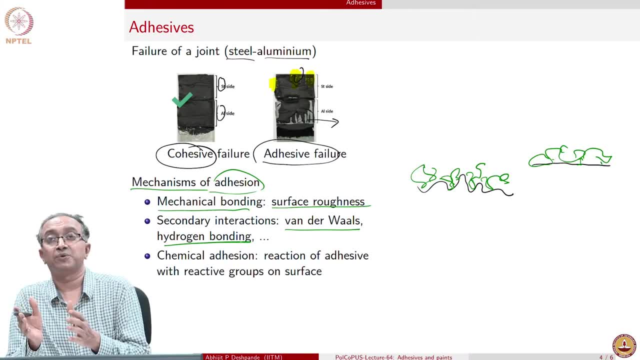 this case, If, let us say, we take two different polymer composites and want to join them, then in that case the macromolecule of the two pieces which are going to be joined and the macromolecules of adhesive. they need to interact with each other using van der Waals or other secondary interactions, as the case may be. 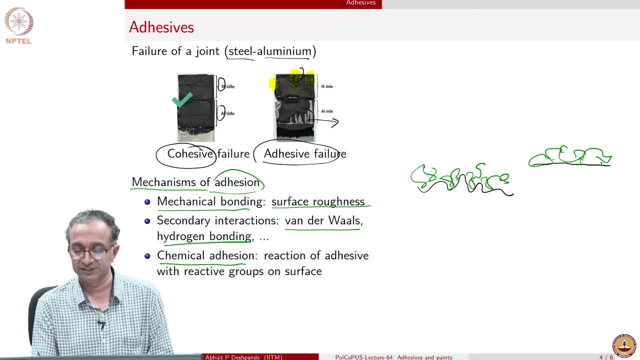 And then of course we can also have chemical adhesion, where this can form covalent bonds or ionic bonds, So that there is a adhesion actually reacts with and reacts with each other, So whatever are the active groups present on the surface, So, depending on the type of adhesives, 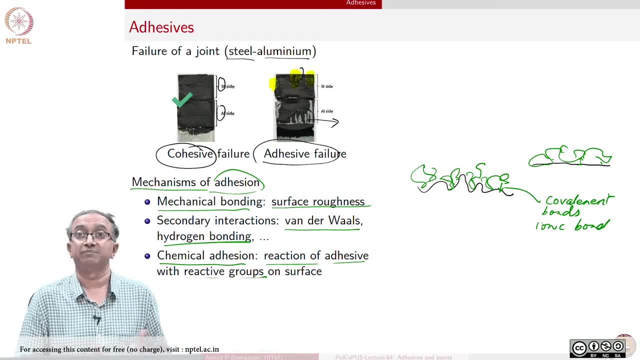 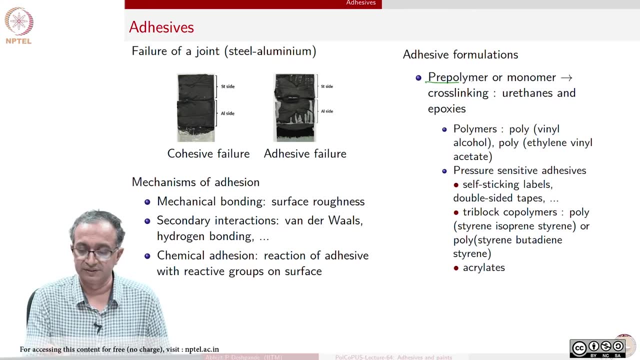 each of these mechanisms, or multiple such mechanisms, can be there in case of a single adhesive, And so generally, adhesive formulations have a pre-polymer or a monomer, and then we have cross-linking going on, because when we need to apply the adhesive, we need sufficient. 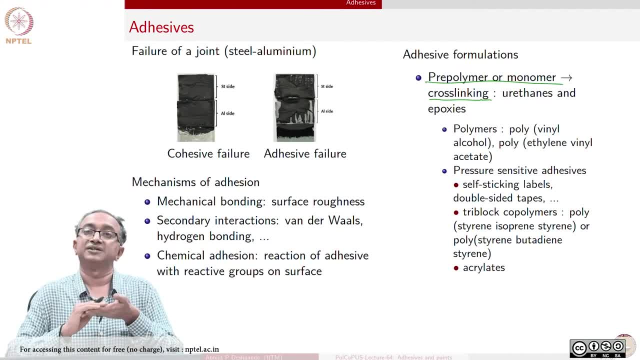 flow behavior. But in the final part, the adhesive needs to be strong, such that it itself has good strength. at the same time, it needs to also form very good bond with the both the surfaces which it is trying to bond, And so with a liquid state, with a pre-polymer or a monomer state. 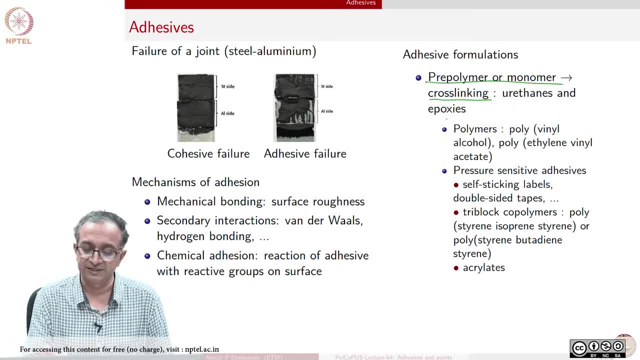 it is easier to do this. So urethanes and cross-link epoxies are quite commonly used as adhesives. We also have polymers such as PVA adhesives and adhesives, So adhesives are quite commonly used as adhesives. 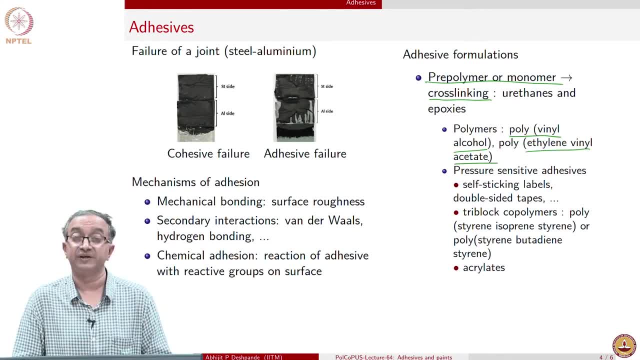 polyvinyl acetate, ethylene vinyl acetate, which are very good adhesives. Some of these can also work as pressure sensitive adhesives, where a lot of these sticky notes and double sided tapes where you remove the backing material and then immediately it can bond. 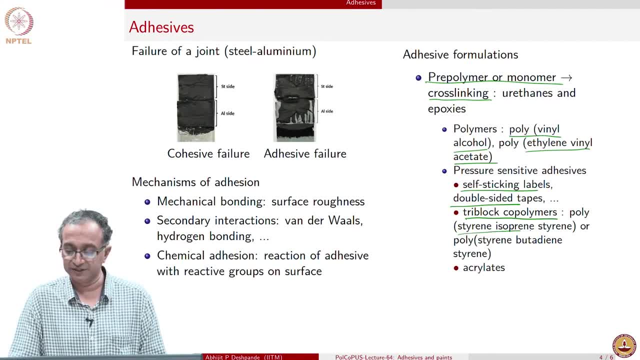 We also have trigoblock copolymers, which are styrene, isoprene styrene or styrene, butadiene styrene, which can act as very good adhesives. What you can see in many of these adhesives cases is a good distribution of polar and non-polar entities And these distribution. 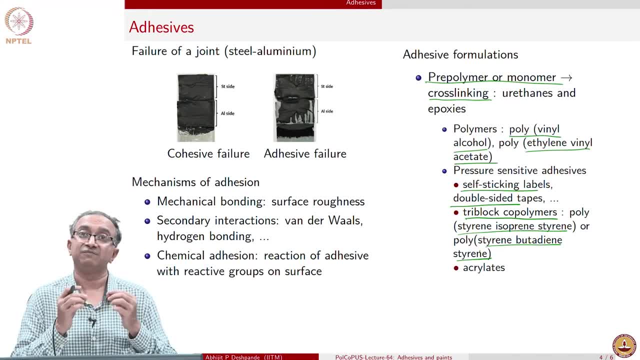 of polar and non-polar entities ensure that there is always sufficient number of points at which this macromolecule can form good interaction with the substrate which it is trying to bind. Now let us look at the other example of a product which where, again, the 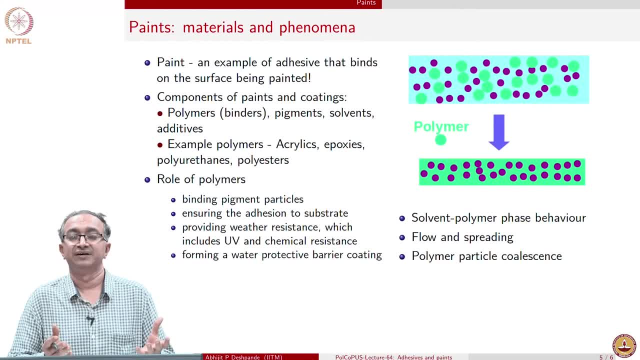 interaction with the other substrate is crucial is paint. Paint is nothing but actually an adhesive which is used to bind adhesives, So paint is used to bind adhesives. So paint is used to bind adhesives binding on the surface being painted. So when we apply a paint, we want the paint. 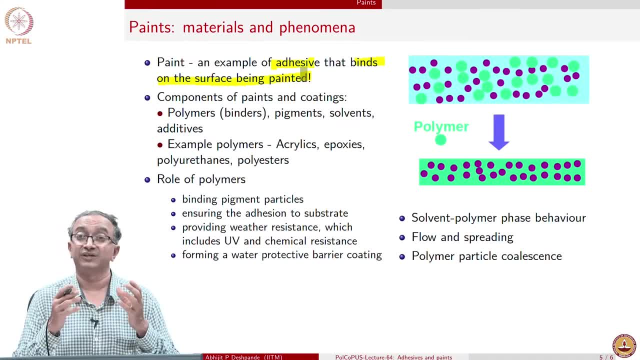 to stick to the surface on which we are applying it. So therefore there is adhesion also involved and at the same time we want the outer surface of the adhesive to give color or any other feature that we want from an aesthetic point of view. We also can do paints and coatings. 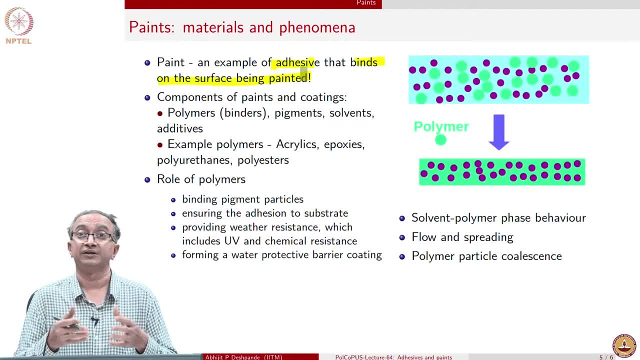 for protecting, in terms of anti-corrosion protection or in terms of scratch proof protection and so on. So paints and coatings can play several roles in addition to being aesthetically giving pleasing surfaces. So general components of paints and coatings are polymers, which 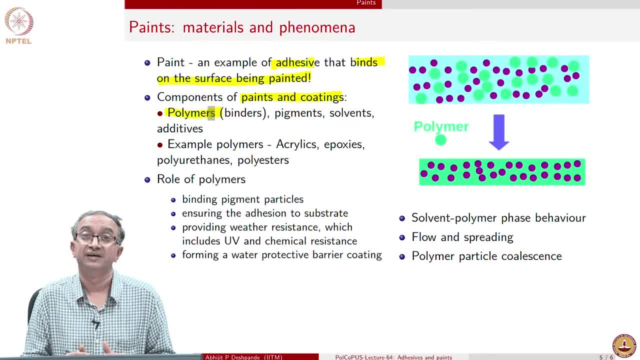 are actually the adhesives and therefore they are called the binders. They also bind the pigment particles together, because quite often paints and coatings may also have colors and pigment particles. So they have to be held together and that is the job of polymer. 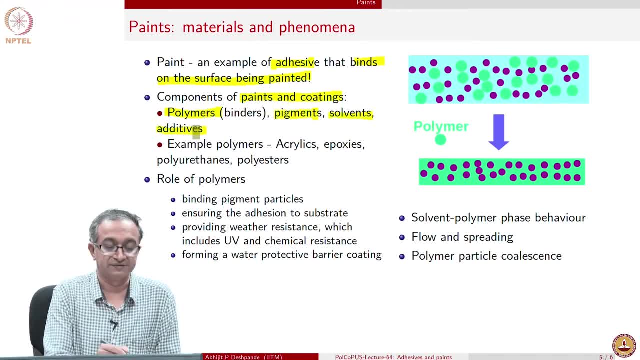 So paints can be there, solvents and additives can be there to make sure that all these multiphase system of polymers particles is remain stable. it is well distributed and the viscosity is nice in the sense that when we are trying to apply the paint it can be applied easily. 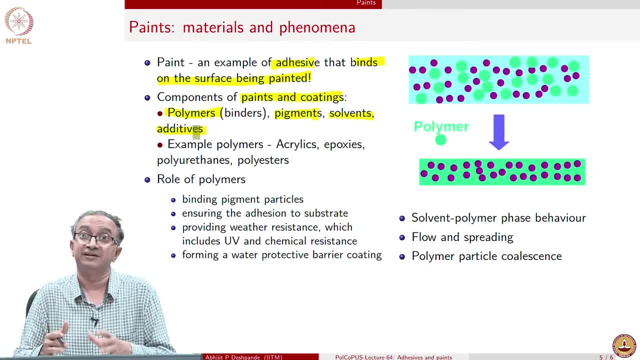 But as soon as we stop applying it, wherever we have applied it, paint stays there. So rheological response of paints is also very crucial in terms of determining its overall resistance And, again, macromolecule plays a very significant role in determining the. 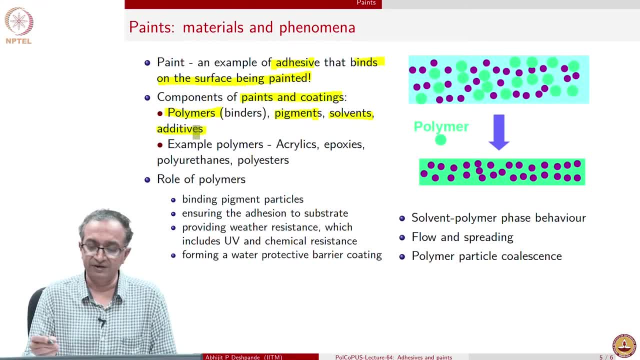 rheology of such paint systems. Effectively, what we have is depicted here. Initially, we start with a paint formulation in which we have these polymer particles and we also have the pigment particles, and then the solvent, which is depicted in blue here, has to disappear. 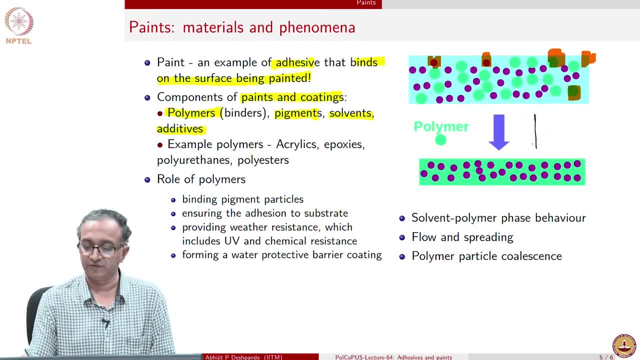 so that when we go to a final paint formulation, the solvent is no longer there, the pigment particles get distributed very nicely and the polymer forms a film. and this polymer film will do two jobs: it will make sure that the pigments are well distributed and it gives 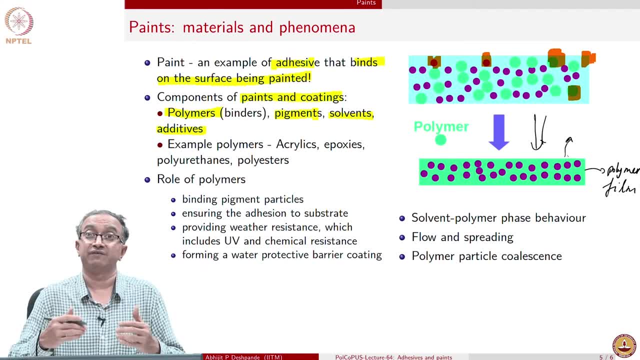 aesthetically pleasing or scratch proof surface or whatever is the functionality on one side and on the other side it gives good addition to the substrate. So therefore, polymers are quite crucial in this application, and general examples of polymers which are used in case of paints are acrylics, epoxies, polyurethanes, polyesters- so many. 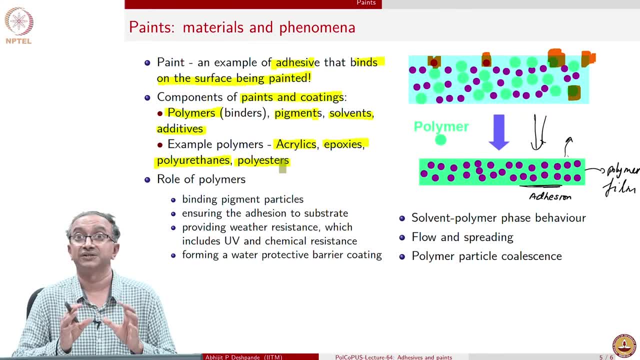 similar polymers, again because adhesion is a very important component of paints and so role of polymers, in summary, is to bind pigment particles, Make sure that there is addition to the substrate. it can provide weather resistance, and which includes UV and chemical resistance, and it can form also water protective barrier coating. 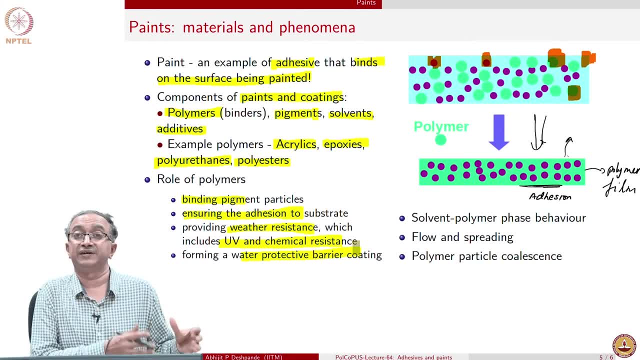 And so in such a system where you are going from a multiphase polymer particle solvent system to finally, a polymer particle system, lot of interesting thermodynamic questions related to miscibility of solvent polymer systems are involved. Thank you very much. In terms of wettability and interface between the spreading paint and the substrate, or how? 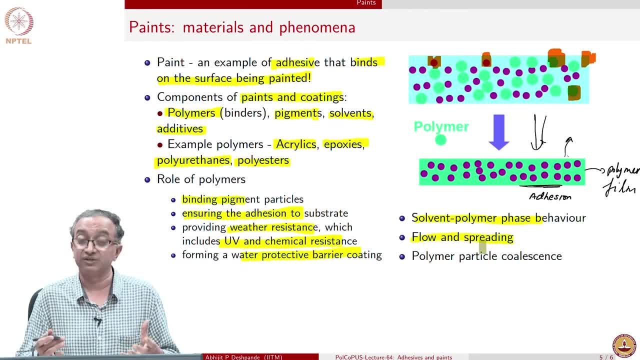 the viscosity and rheology of this paint is. these are also very important. and finally, how do these green polymer particle come together and then finally lead to a very uniform film? So, polymer particle, coalescence and formation of a film, these are all very fundamental phenomena. 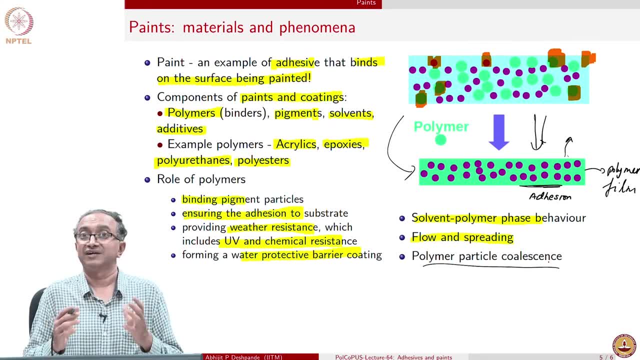 which happen during a painting process. Fascinating, isn't it? I mean, When we think of it, we just think we are applying a paint and then it just forms a very nice film. But if you look at it from the point of view of thermodynamics and kinetics of the processes, 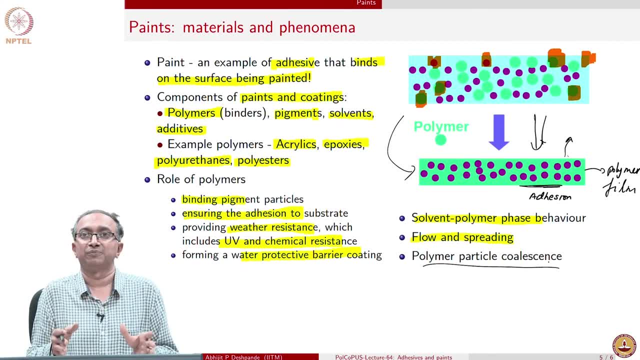 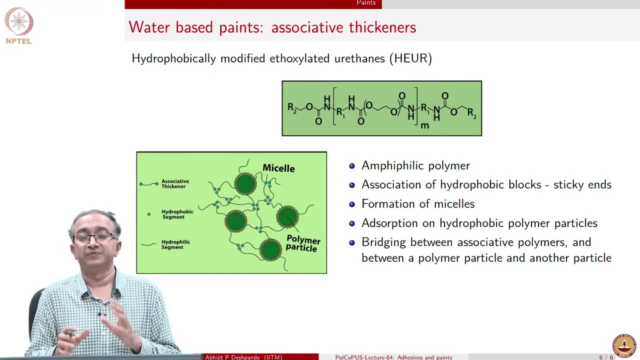 which are happening, lot of role of macro-molecular phenomena in terms of performance of a paint system To leave you with an excellent- again- example of how interactions are manipulated to devise an excellent paint. There is a lot of emphasis on water-based paints so that when solvent evaporates it. 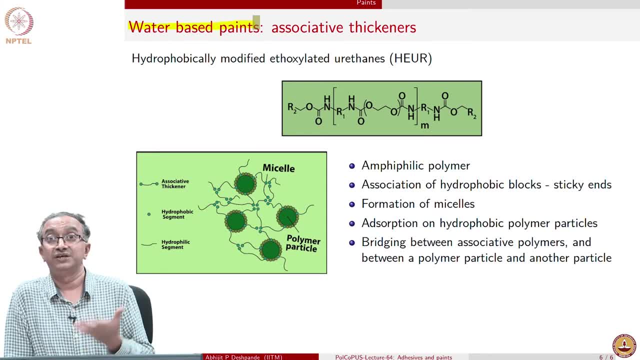 does not have an environmental impact. So the emulsion paints. many times you might have heard, and then they will say water-based emulsions, And so whatever is evaporating in this case is just water, And so water-based paints are using these days what are called associative thickeners. 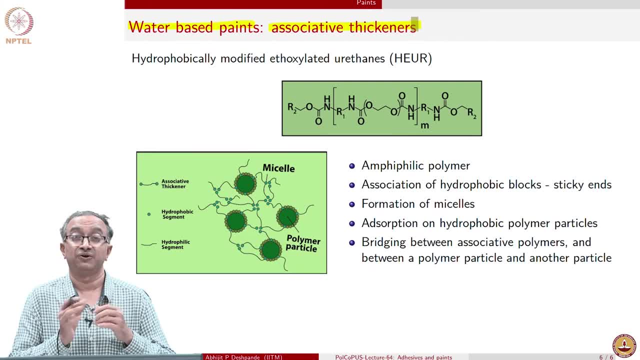 So, as the name suggests, thickeners, they modify the viscosity and rheology of the material, And they do this by associating. And what do we mean by that? So what we have these are basically urethanes, but they are ethoxylated. 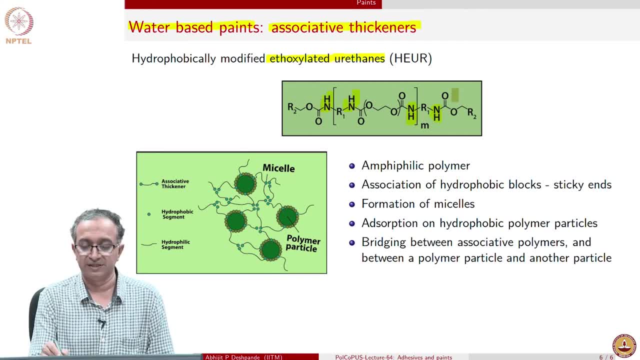 So there is all these urethane linkages, but there are several ethoxy groups also, And because of these kind of variated groups on them, the ends of these macromolecules become sticky. So what you have effectively is a macromolecule which is like this: 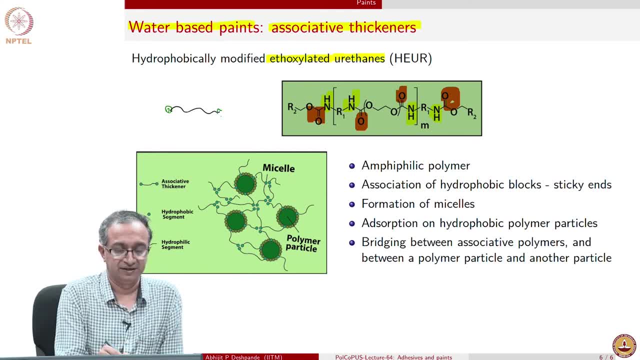 It has a hydrophobic modification at the end and then overall it may be hydrophilic. because of these R1 and R2 groups And because of this, if you put another molecule of this together, the green and green part would like to come together. 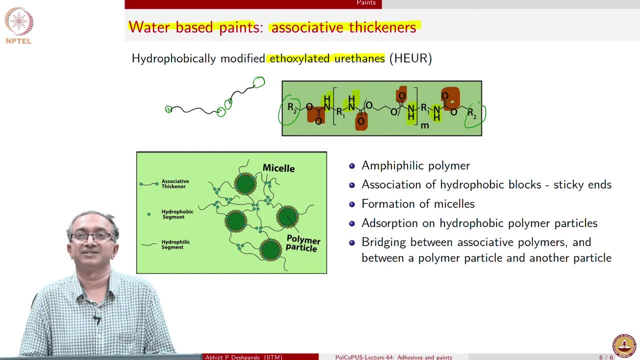 So therefore, there is an association between hydrophobic parts- This can also be called sticky polymers, And they have polymers with sticky ends, So the ends which are sticky would like to stick with each other. And so, if you look at closely, what is the system in the end? is you have a polymer particle. 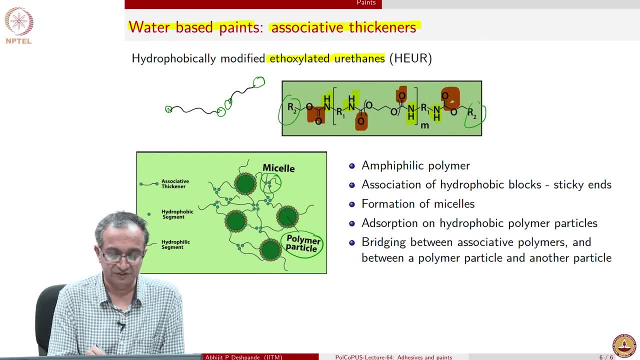 and then you have complex structure which is formed by these sticky polymers, So they can form micellar-like structure, They can bond with the polymer particle And by doing this they are forming a three-dimensional network. And we have of course discussed 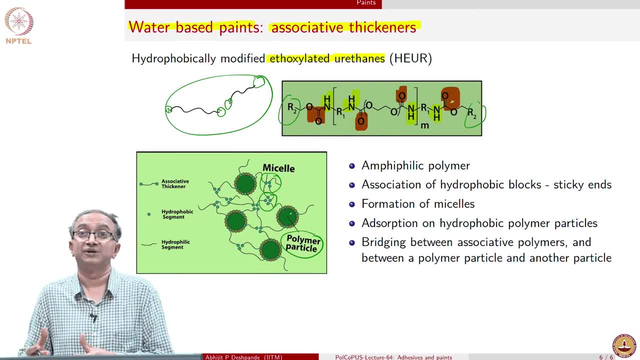 In case of polymers, how formation of a three-dimensional network leads to very complex behavior And you can of course always reach the gel or more solid-like properties. So in this case also, thickening action and rheology modification happens because of this. 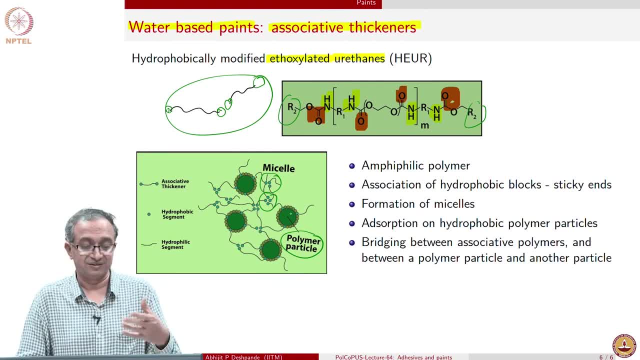 network formation. The interesting thing here is this network is being formed based on physical bonding stickiness of hydrophobic parts of a macromolecule. So generally these associative thickeners are amphiphilic Polymers because they have this green hydrophobic part and the black hydrophilic part and the 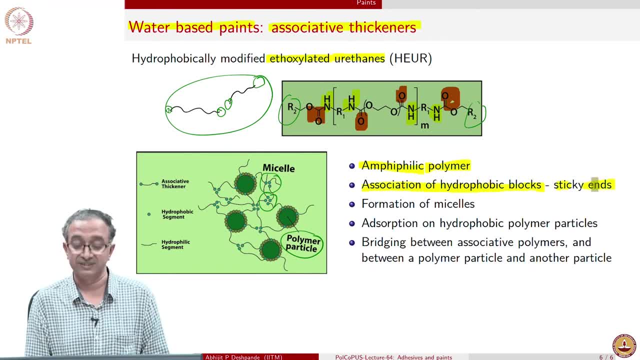 association of hydrophobic blocks leads to what are called the sticky ends, And then these could lead to micelles. They could adsorb on the polymer particles and they act as bridges and form the three-dimensional network. So you can read more about these paints, which include these hydrophobically modified sticky.